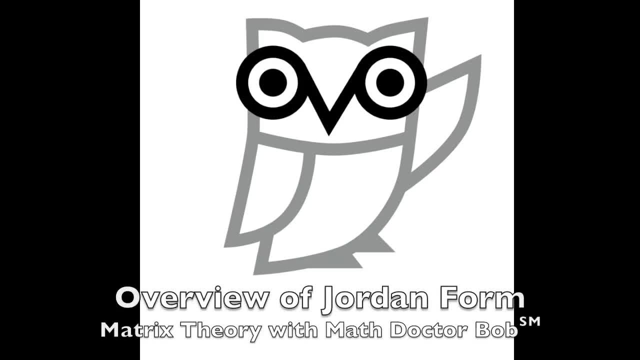 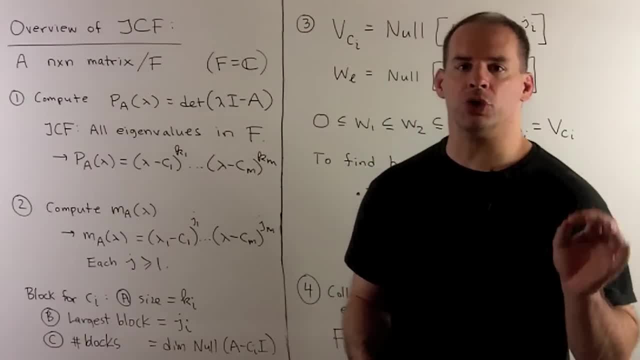 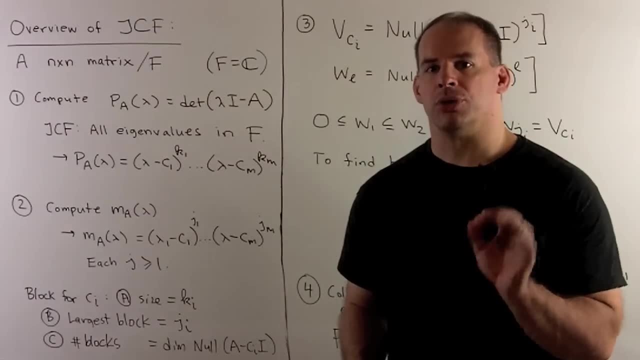 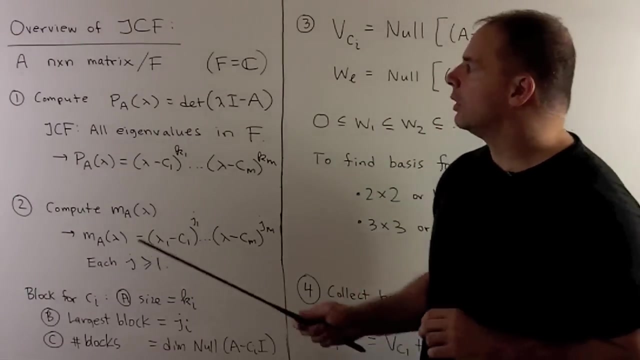 Here's an overview of a Jordan canonical form. We'll break the examples out over several videos. Here we'll just give one example. that gives a general flavor of the big picture. Now we'll have n by n, matrix A over some field, F. F is the complex numbers We can. 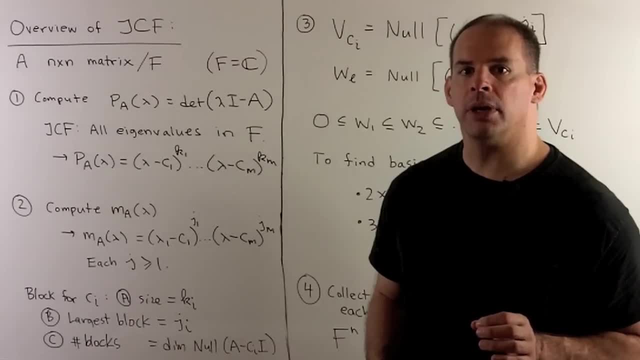 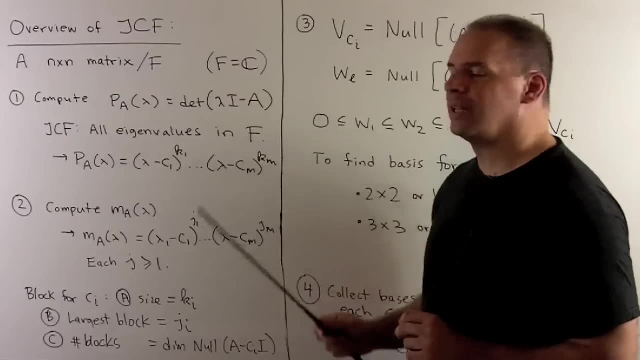 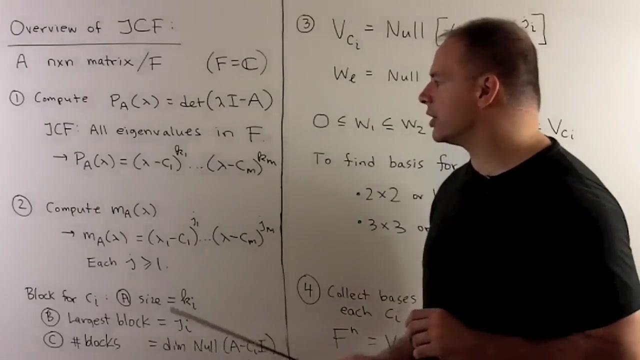 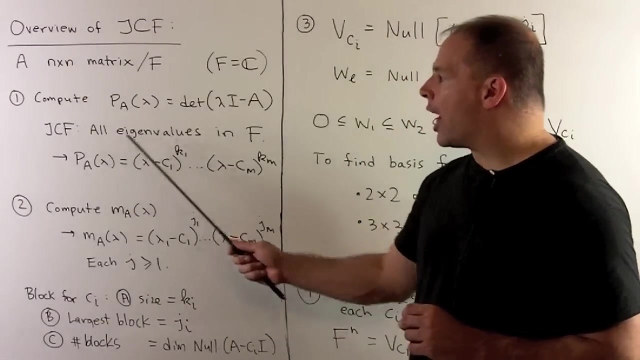 always put our matrix A in Jordan canonical form. We start by computing the characteristic polynomial of A, So it's determinant lambda I minus A. If we could factor the characteristic polynomial completely into powers of linear factors, then we can use Jordan canonical form Another way to say that all eigenvalues are going to live in our base field. Now 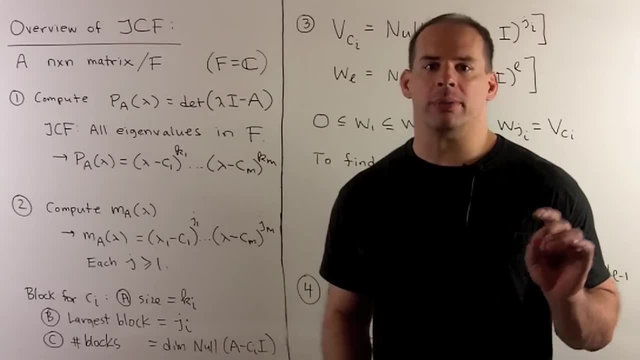 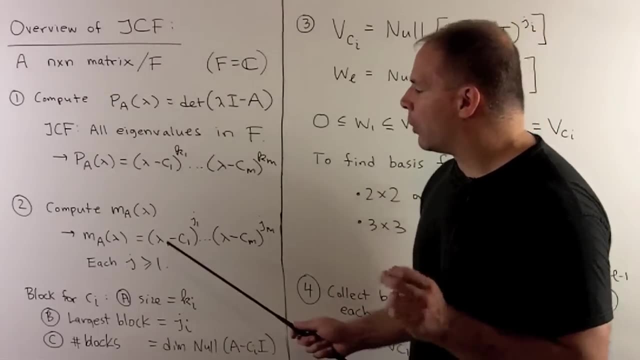 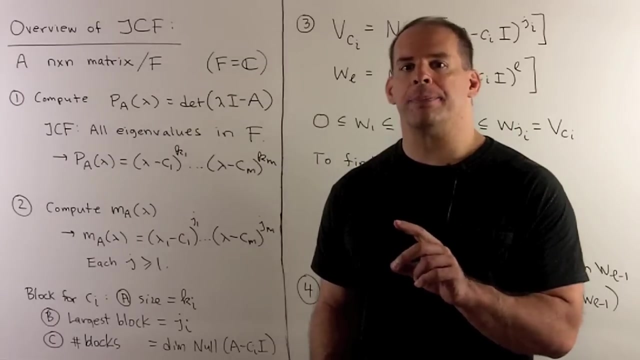 if this condition fails, then we have to use another canonical form, such as rational canonical form. Once we have our characteristic polynomial, I want to compute the minimal polynomial of A. This will be the monic polynomial of smallest degree, such that if we evaluated A as a matrix, 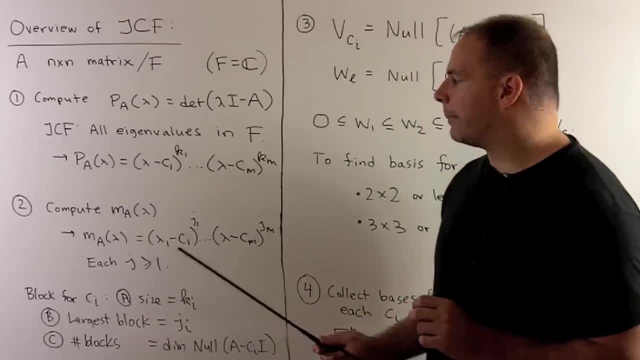 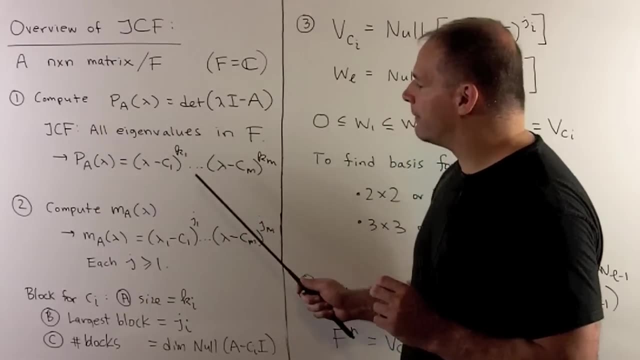 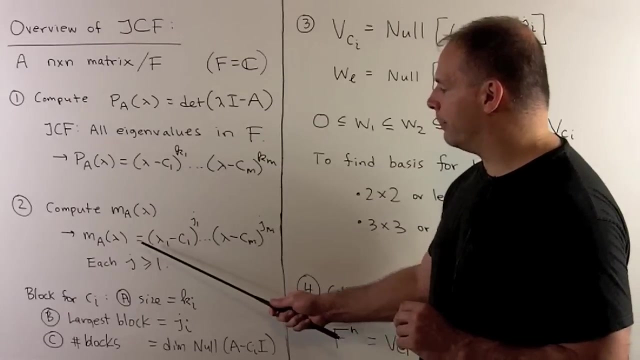 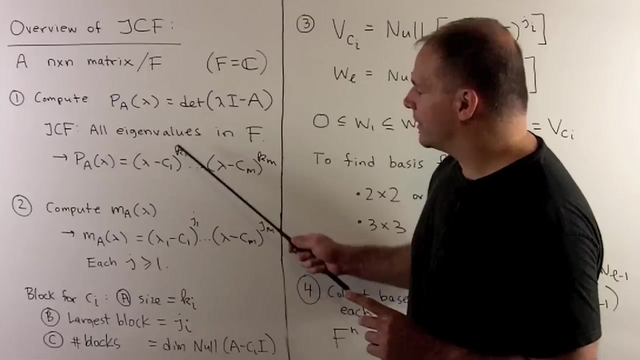 polynomial we get the zero matrix out. Now we know the minimal polynomial of A divides the characteristic polynomial of A and if we have some factor that occurs in the characteristic polynomial, that irreducible factor must occur in the minimal polynomial with degree at least one. So only difference here: we have the same factors but we may have different. 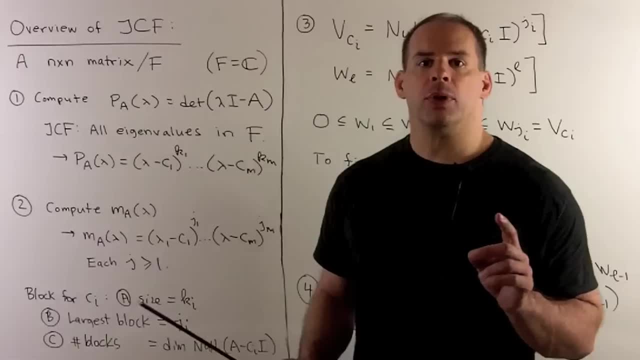 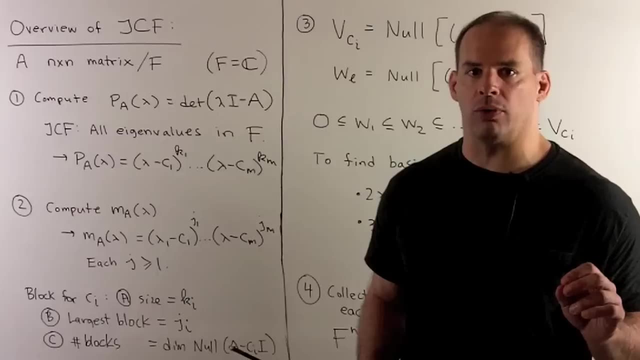 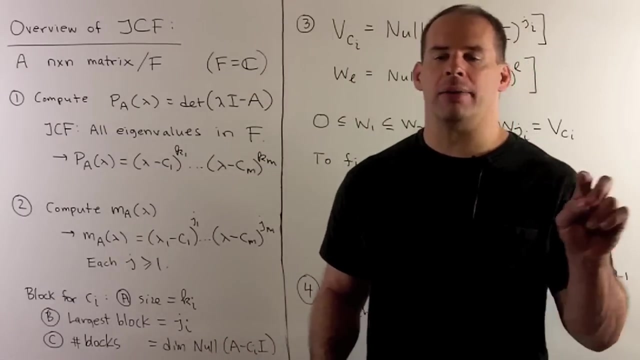 exponents. Now, with these two polynomials we can get some data that gives us crude information about our Jordan canonical form. So if we fix an eigenvalue, C sub i, we're going to focus on the block for C sub i. This block is going to be composed of Jordan blocks going 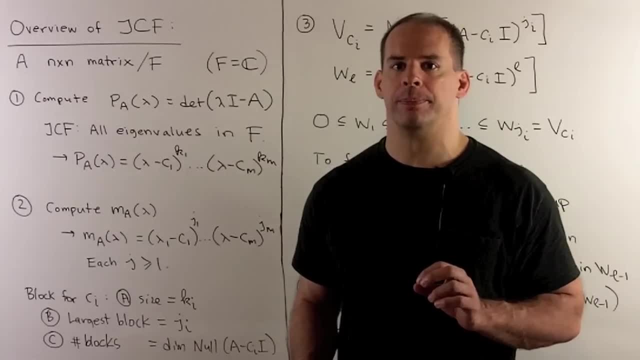 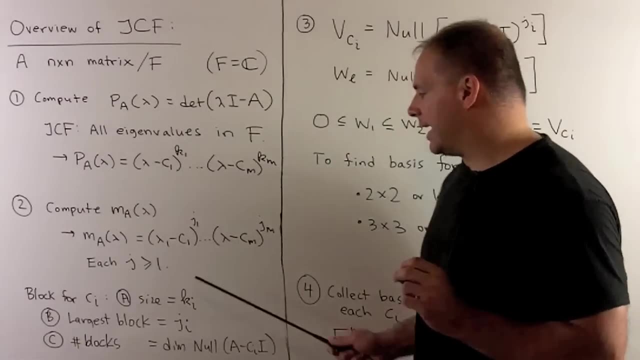 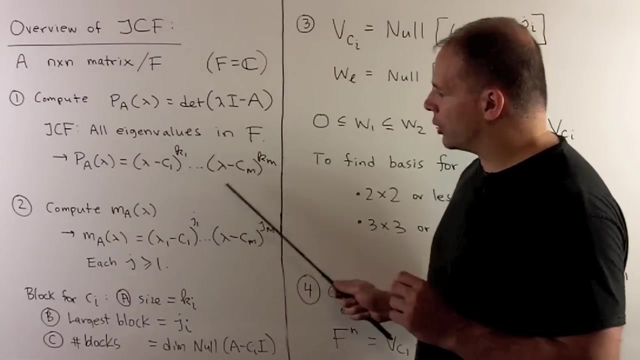 down the diagonal. We'll talk about Jordan blocks in a little bit. The size of the diagonal is going to be the size of all of our blocks put together. It's going to be equal to K sub i. K sub i is going to be the exponent of lambda minus C sub i in our characteristic. 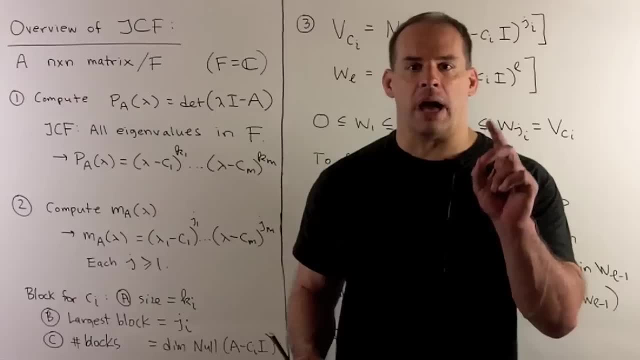 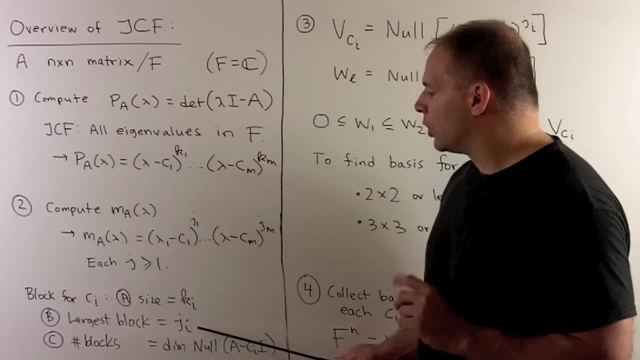 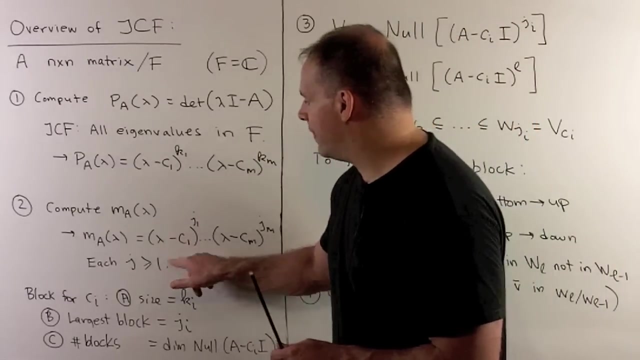 polynomial. Now, looking at the Jordan blocks, going down the diagonal, the largest Jordan block is going to have size J sub i, where J sub i is the exponent of lambda minus C sub i in our minimal polynomial. And then if I want to know the number of blocks that go with C sub i, so the number, 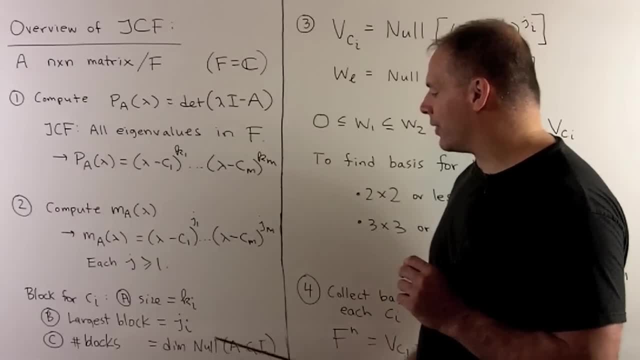 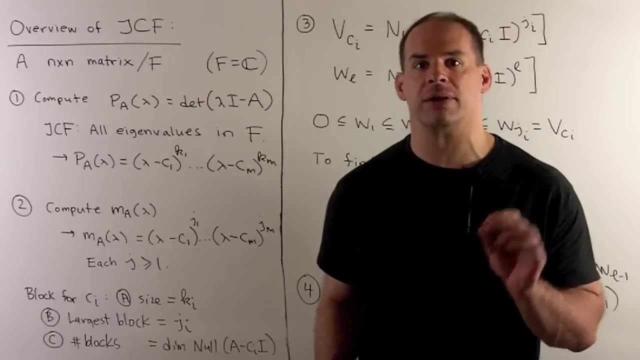 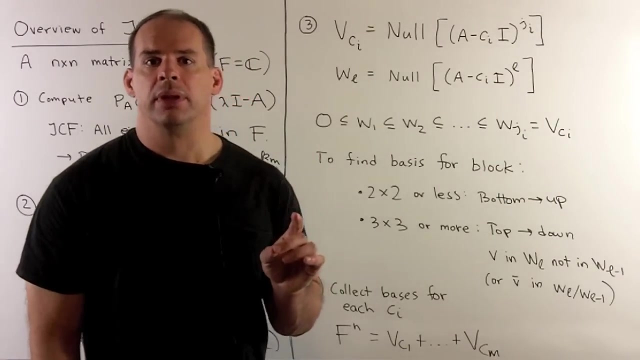 of Jordan blocks, then we're just going to calculate the dimension of the null space of A minus C sub i times i. Okay, this is just going to be the dimension of the eigenspace for C sub i. If I want more information about our blocks or if I want to find a basis that puts A in, 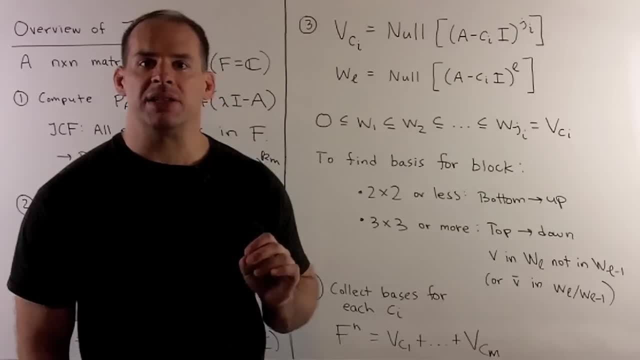 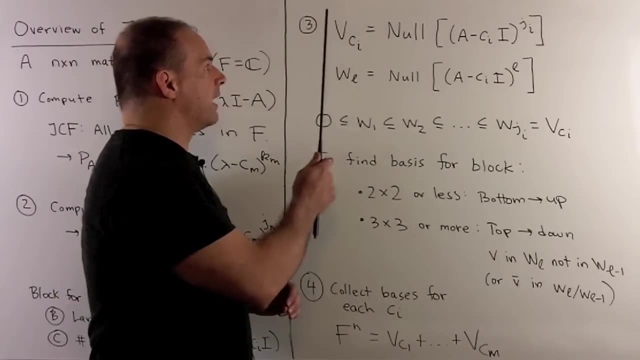 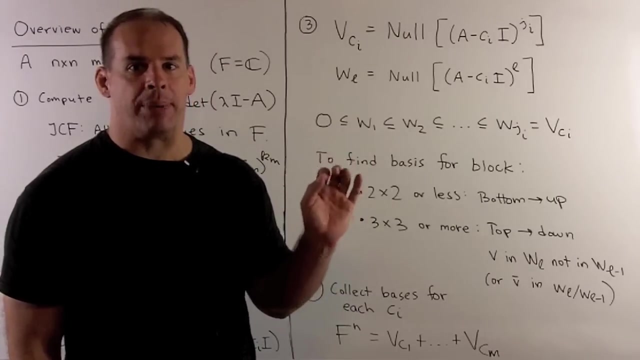 Jordan canonical form. we need to look at null spaces beyond our eigenspaces. So if we fix an eigenvalue, C sub i, I'll define V sub C sub i as the null space of A minus C sub i times the identity matrix raised to the J sub i power. So we'll call J sub i as. 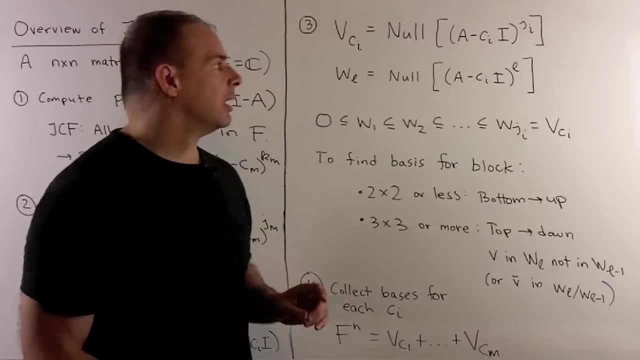 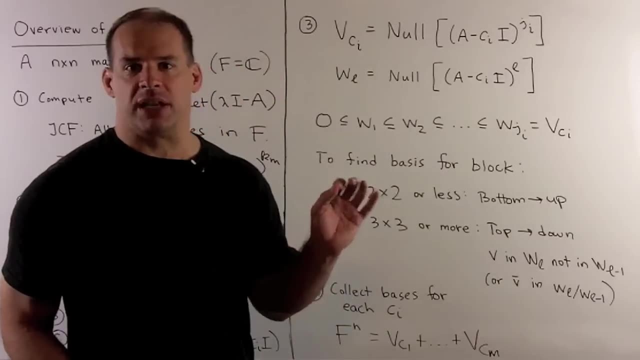 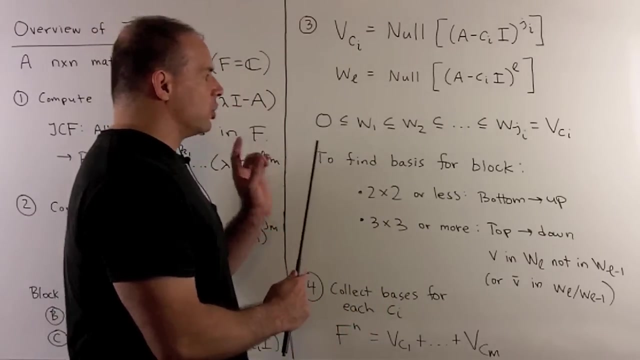 the exponent from the minimal polynomial, Then with C sub i understood we'll define W sub l as the null space of A minus C sub i times the identity matrix raised to the J sub i power. Now this is going to give us a chain of inclusions. so 0 contained in W sub 1, contained 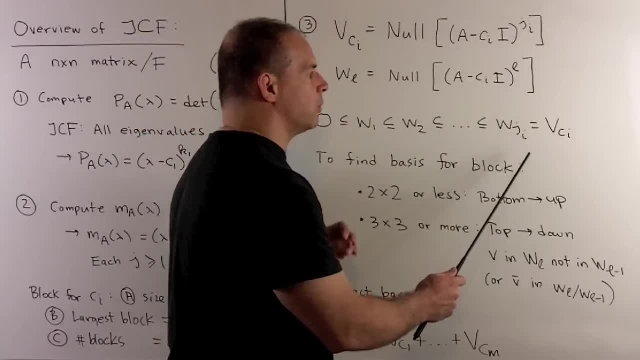 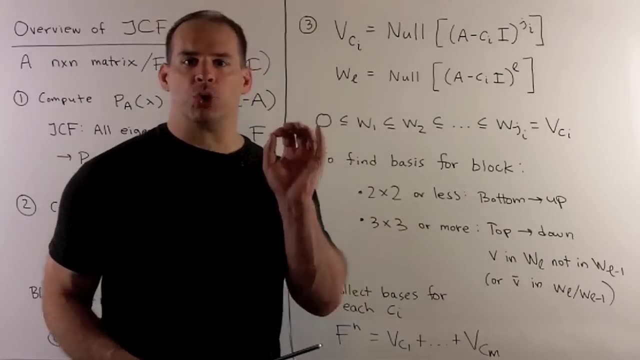 in W sub 2, all the way up through W sub J sub i, which is equal to V sub C sub i. So all the information that we'll need for the block composed of Jordan blocks that go with C sub i is contained in here. 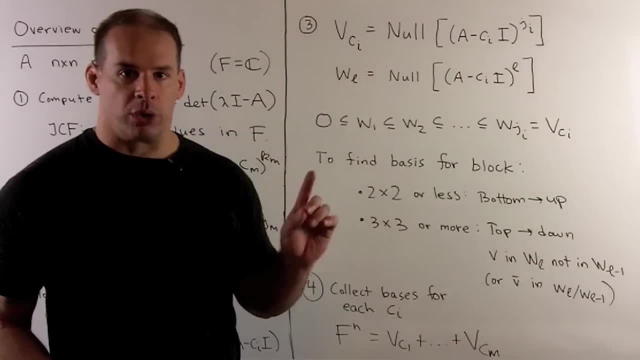 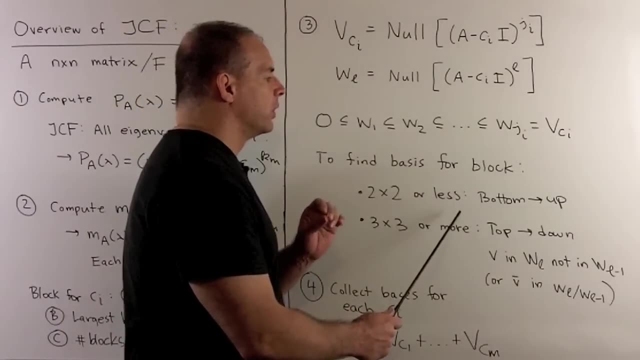 Now, if I want to find a basis for each Jordan block, I'm going to have to find the null space for each Jordan block. Two options: If all of our Jordan blocks are sized 2 by 2 or less, we can work from the bottom up. 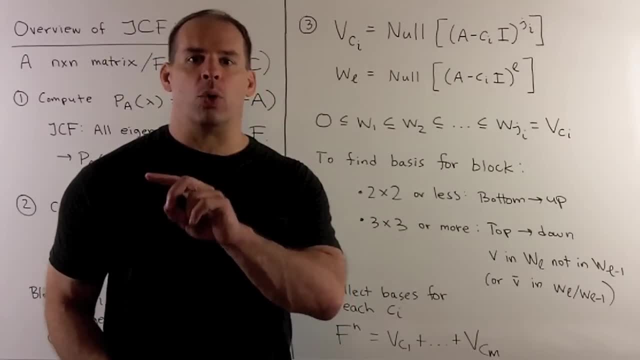 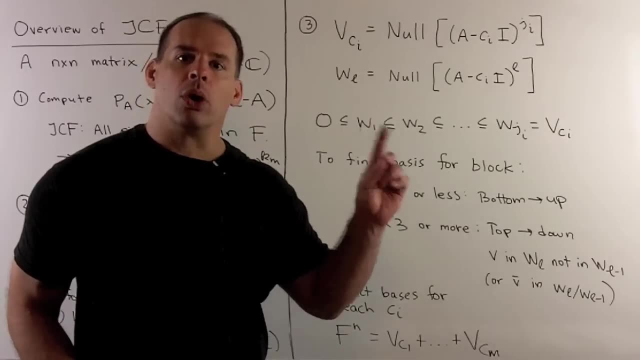 So I could start from the eigenspace and then solve the equations to get to the next level up. If we have a block of size 3 by 3 or greater, then we're going to want to work from the top down. 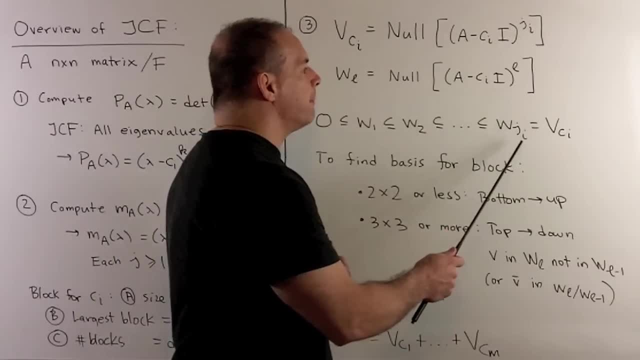 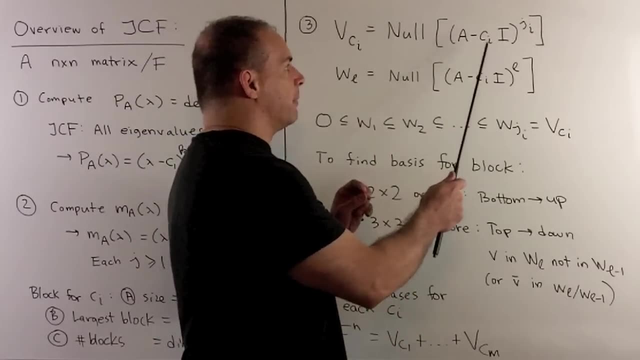 So I would start by finding a vector in W sub J sub i that's not in W sub J sub i minus 1.. We keep applying A minus C sub i i to it, so I can do that J sub i minus 1 times. 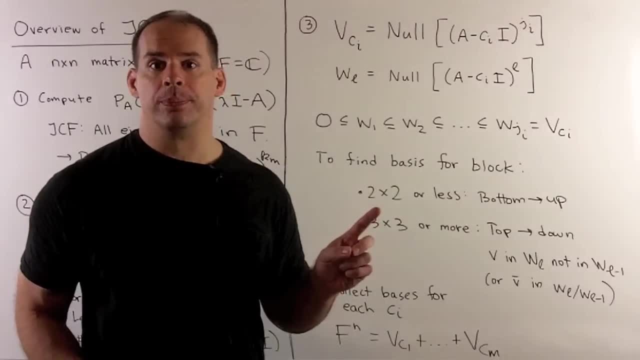 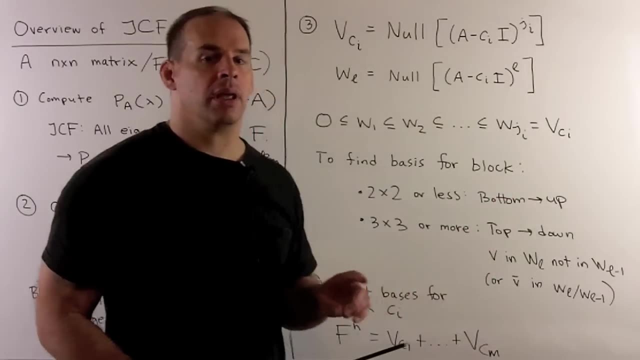 Then on the J sub, i time it's going to send it to 0. That's going to give me a basis for our block, and then we just set those vectors aside. Then we keep repeating until we exhaust all of this subspace that's not in here, and then 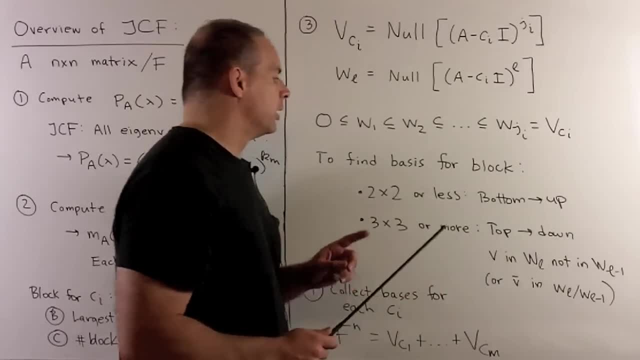 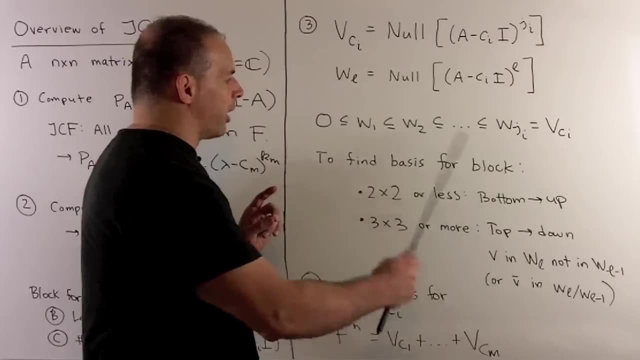 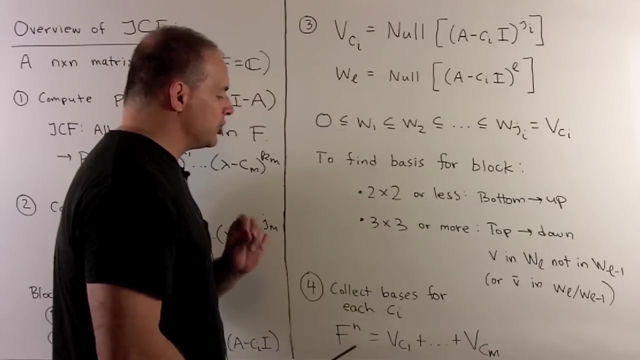 we keep working our way down. Once we've done that, for each eigenvalue C, sub i, we can collect all the bases that we generate from this step. We can put those together and then we're going to have that. our space is just a direct 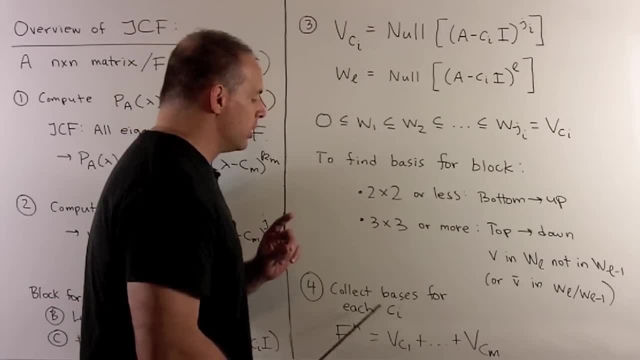 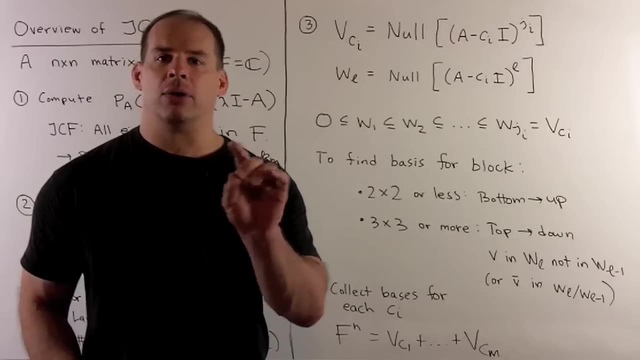 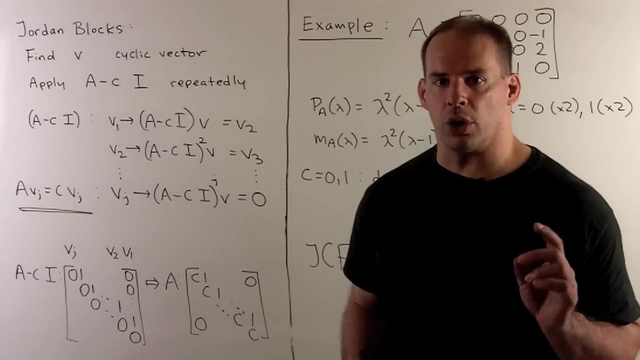 sum of each of our V, sub C, sub i's. So collecting all these bases is going to give us a basis for our big space. Then we just apply our conjugation to get Jordan canonical form. Let's take a closer look at our Jordan blocks. 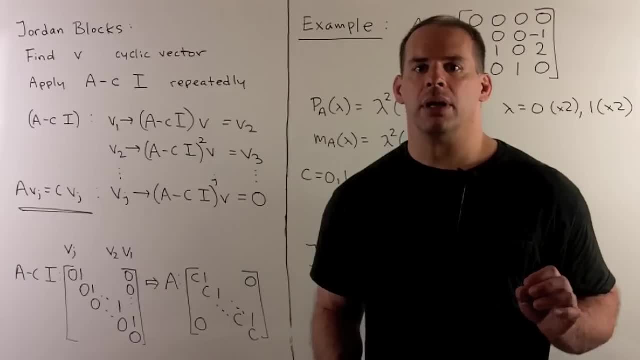 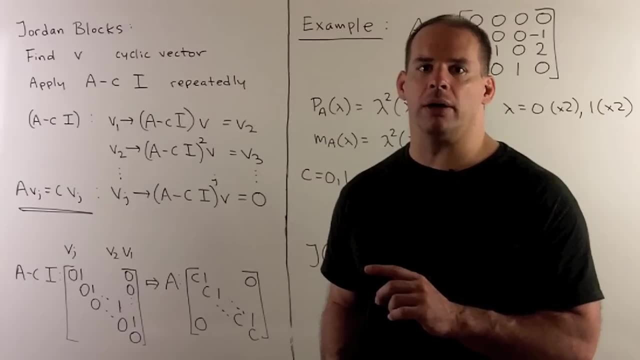 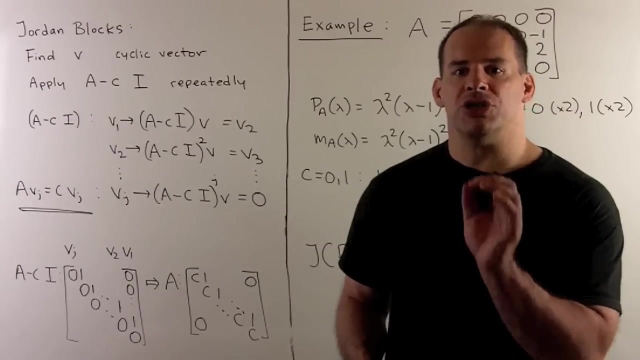 So we'll assume we have a V, as in the previous board. For simplicity we'll assume that V is in the top level. So V is in W sub J, but not in W sub J minus 1.. That means we can apply A minus C, i to V repeatedly, J minus 1 or fewer times to get something. 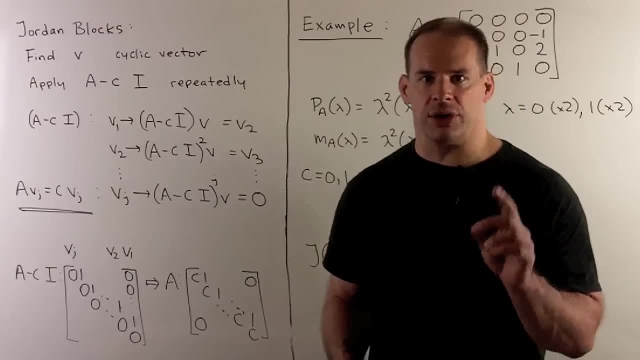 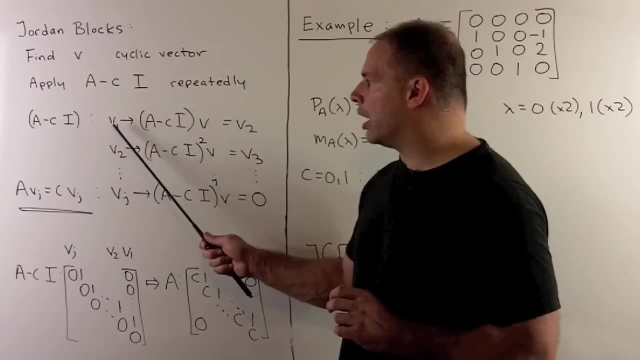 not in 0,, but if we apply it J times, we get 0.. That's how we're going to get the basis that goes with Jordan. That's how we're going to get the basis that goes with our block. So we'll start with V, call it V1. 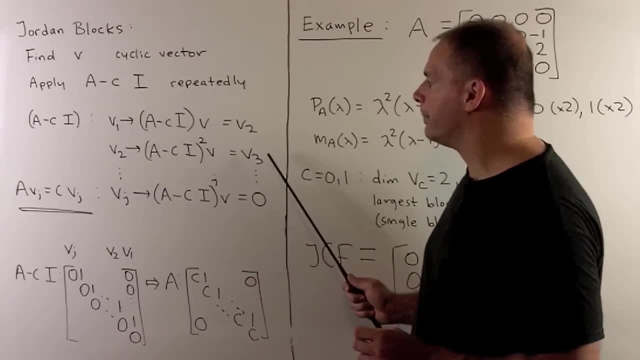 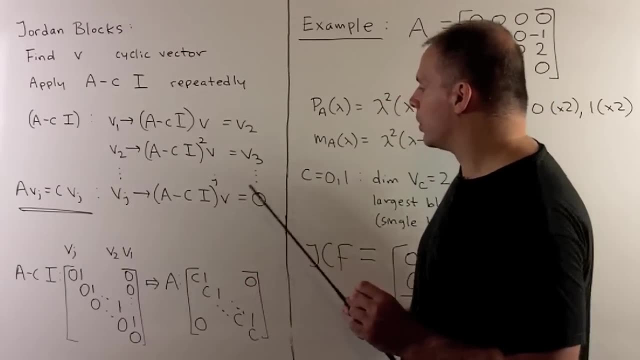 We apply A minus C, i, we get V2.. We apply it again, we get V3.. I could do it J minus 1 times to get V sub J, but if we do it one more time, we're going to send V sub J to 0.. 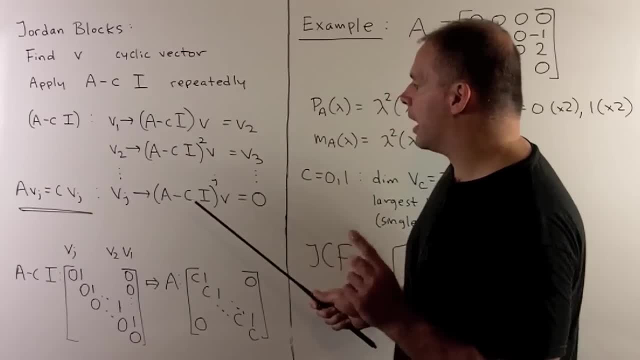 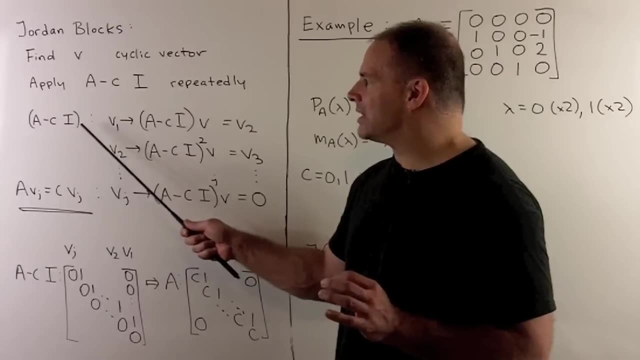 So that's going to be the basis we use for our block. Now one thing to note: okay, V sub J is going to be an eigenvector for A. If we apply A minus C, i to V sub J, we get 0. 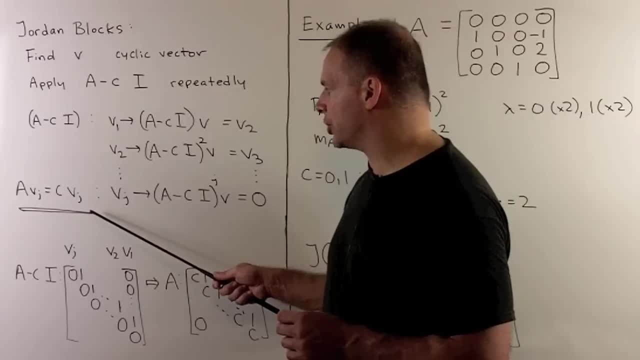 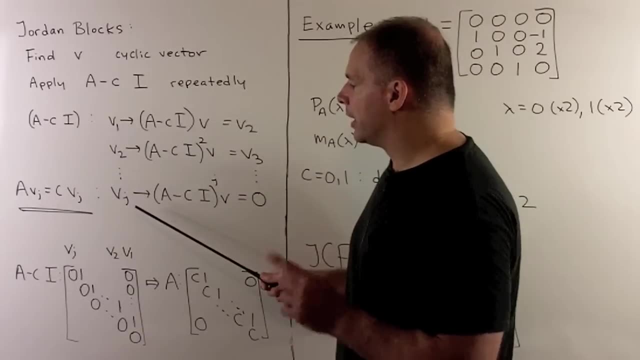 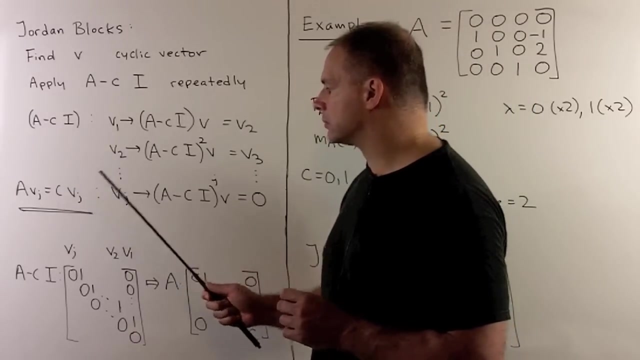 If we push C, V, J to the other side, we have our eigenvector condition. Now note, if we take the span of these vectors, okay, we're only going to have a one-dimensional eigenspace for A with eigenvalue C. 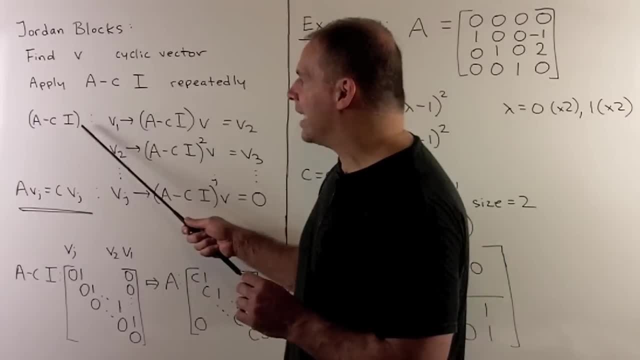 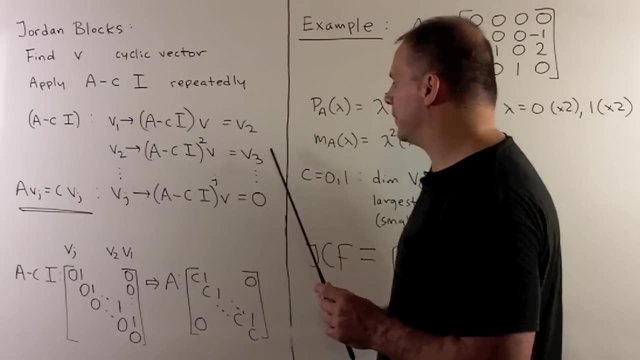 Now, what does A minus C? i look like on this basis. So what's happening? Well, we're going to carry V1 to V2, V2 to V3, V3 to V4, until we get up to VJ, and then 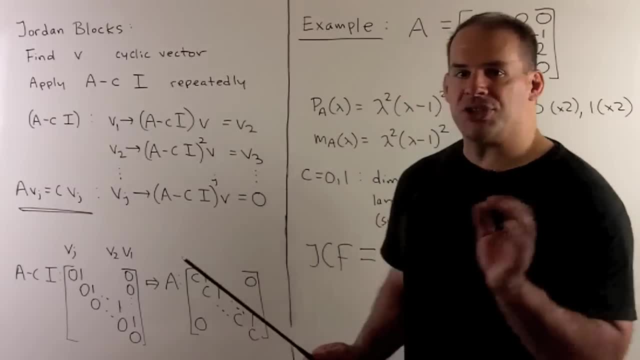 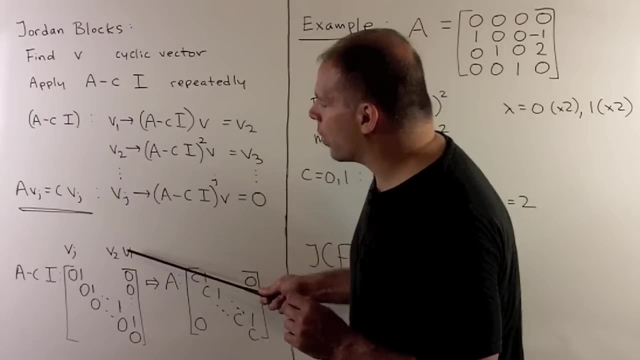 that's going to go to 0.. So, since I like my Jordan form, an upper triangular form, we're going to take our V, put it in the last slot and then we're going to work our way to the left. 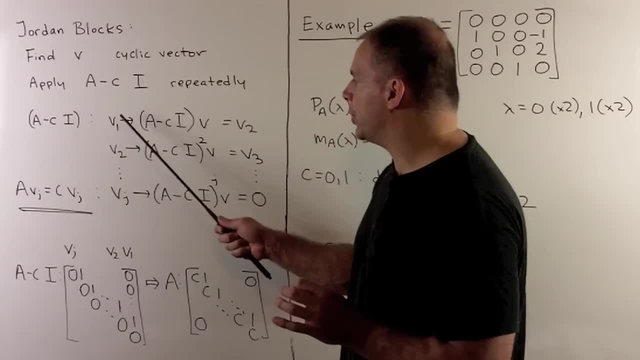 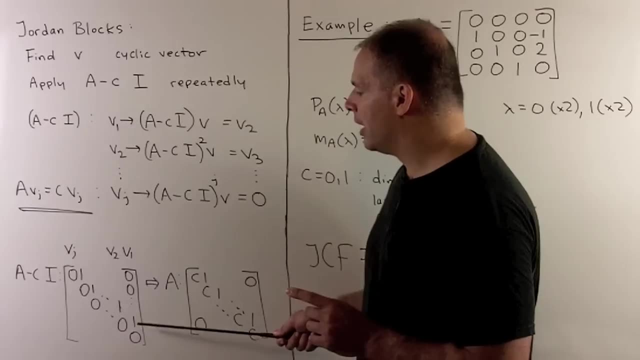 So where does V1 get sent to? It gets sent to V2.. V1 is going to be the last vector, so it corresponds to this 0. in the linear combination, This 1, here 1 corresponds to V2, and then the rest are 0s. 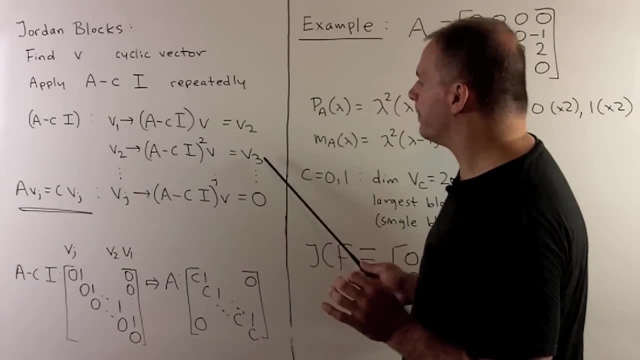 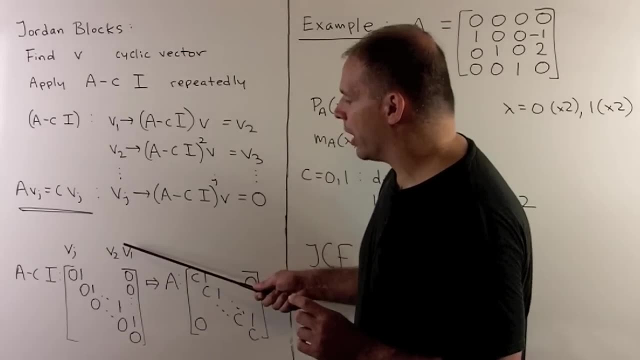 Where does V2 go to? That gets sent to V3. So V1 gets a 0, V2 gets a 0, V3 gets a 1, and then it's all 0s going up. Then you'll see, when we fill everything in, we're going to have 0s everywhere. 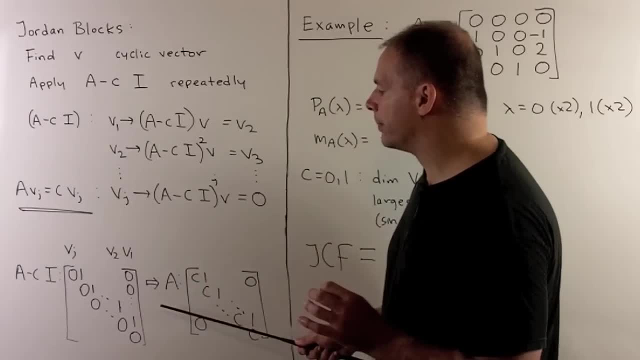 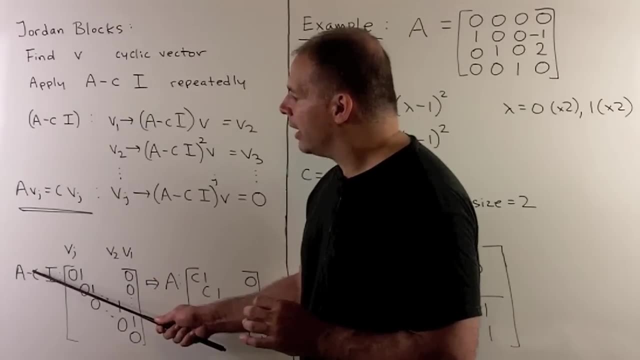 except for 1s on the diagonal, above the main diagonal. Now, if I want to just put this in terms of how A acts, well, if I want to move this Ci to this side, then what we're doing is just putting Cs on the diagonal. 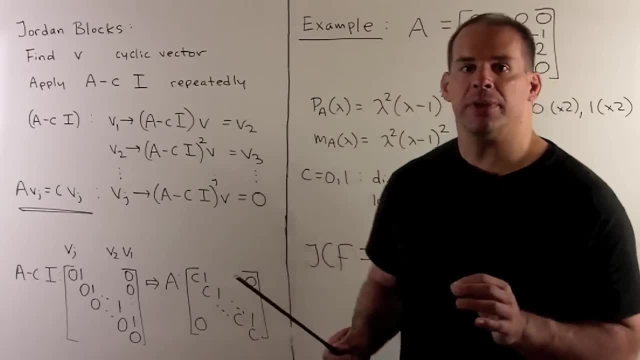 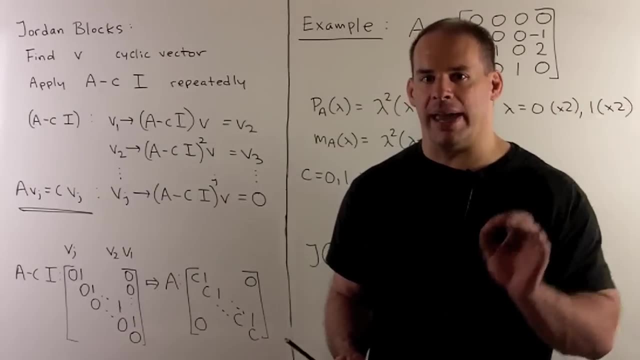 So note, that's what our Jordan block looks like. It's going to be 0s everywhere, 1s on the diagonal, above the main diagonal, and then C your eigenvalue, down the main diagonal, If you like. your Jordan form, lower triangular. 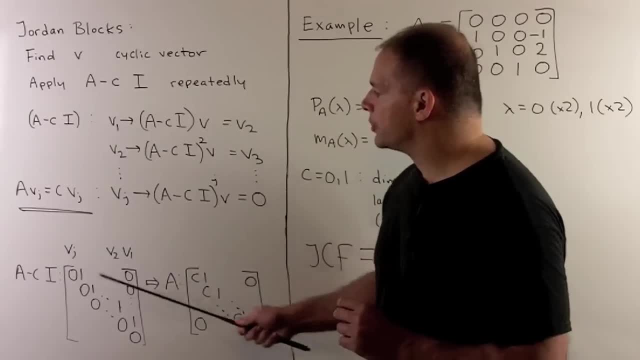 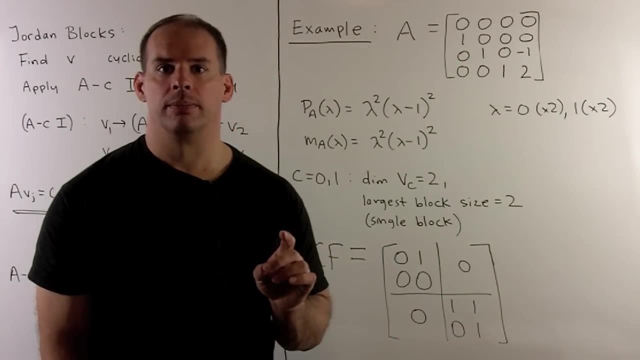 then you're just going to put your basis vectors in the other order. So I start with a V1, and then I work my way to the right. Finally an example. So in this case we'll have two eigenvalues. 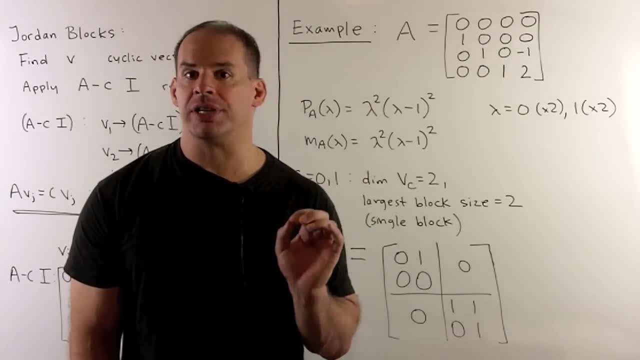 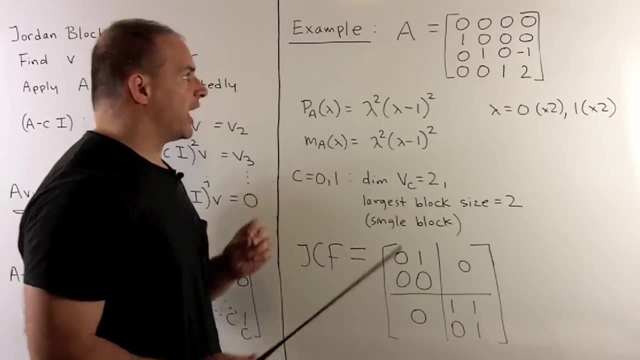 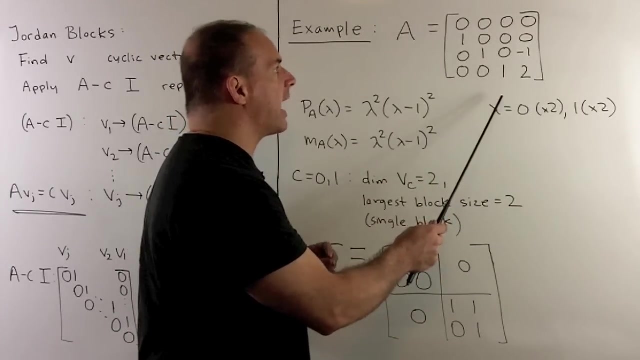 So we'll have two Vs. Each V is going to consist of a single block. Then we'll find the generator for each block. Now our matrix A: get over the complex numbers. We have 0s everywhere, except for 1s on the diagonal below the main diagonal. 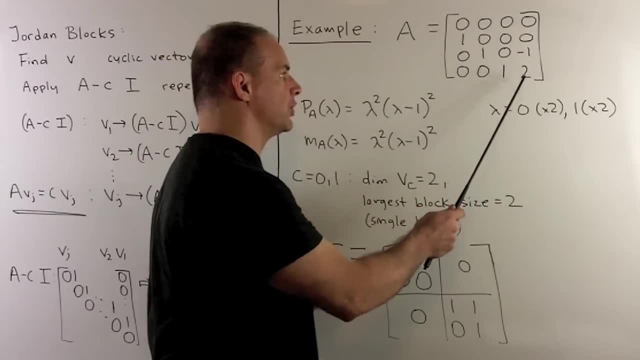 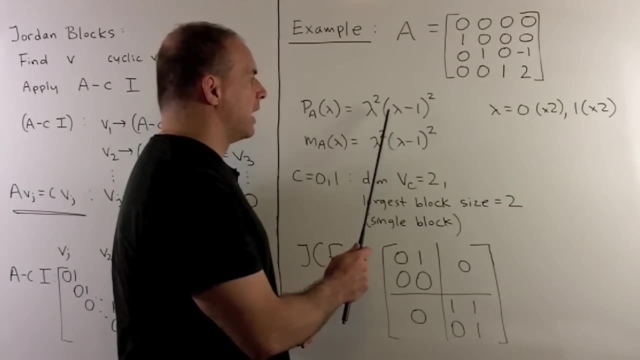 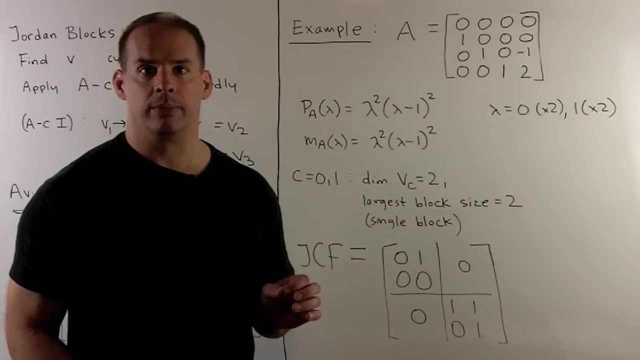 In the last column I have 0, 0, minus 1, 2.. We work out the characteristic polynomial. We'll have lambda squared times lambda minus 1 squared. So our eigenvalues are 0 and 1, each with multiplicity 2.. 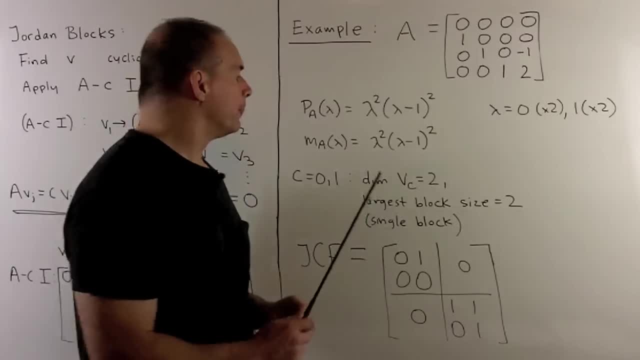 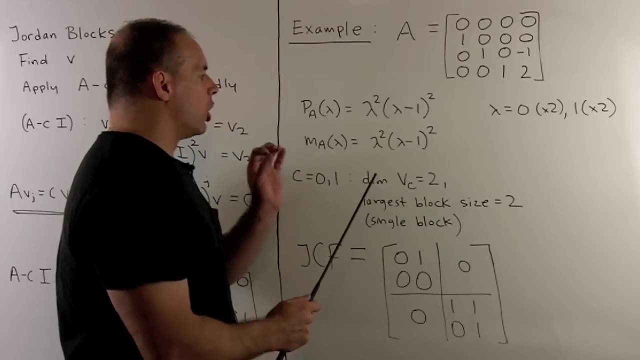 For our minimal polynomial. okay, so that you have to work out. we'll have lambda squared, lambda minus 1 squared, So these are equal. And now we see the largest block for eigenvalue 0 and eigenvalue 1,. 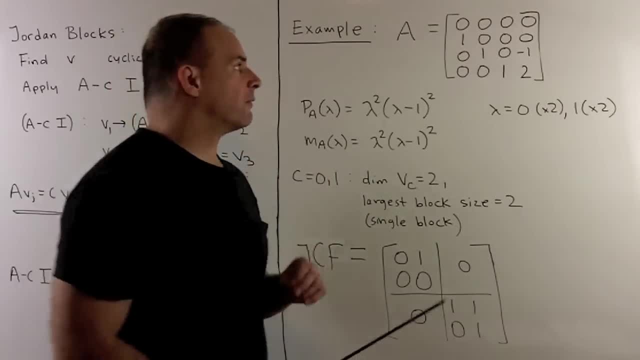 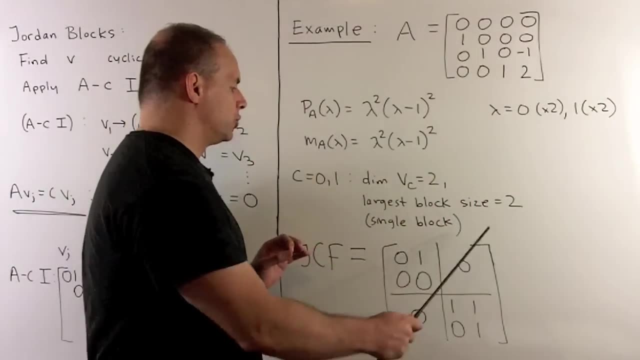 are both going to be equal to 2.. Since I have a 4 by 4 matrix that gives away our entire Jordan canonical form, We're going to have two blocks. Okay, the dimension of each V is going to be equal to 2.. 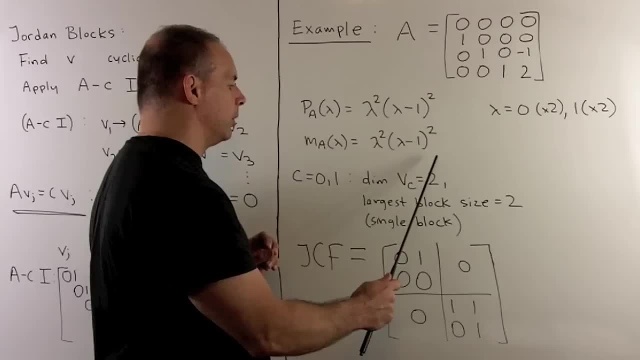 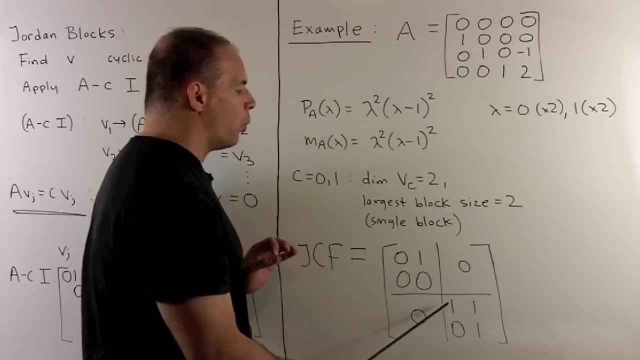 We have a largest block, of size 2, by that minimal polynomial. So we see that we have to have the Jordan form. Okay, 0, 1, 0, 0 for the 0 block. 1, 1, 0, 1 for the 1 block. 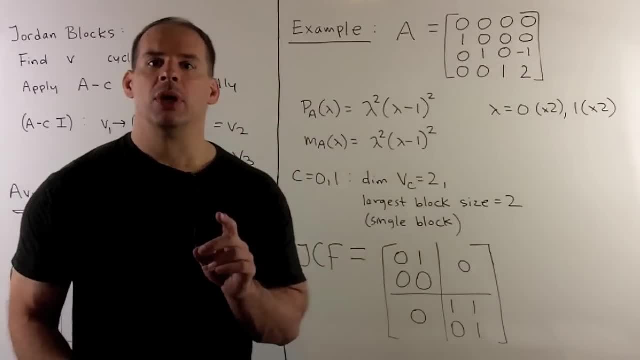 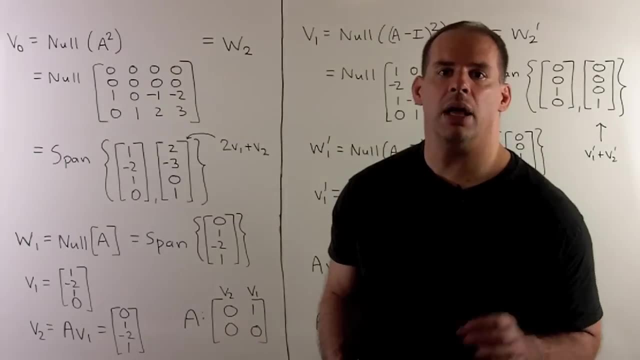 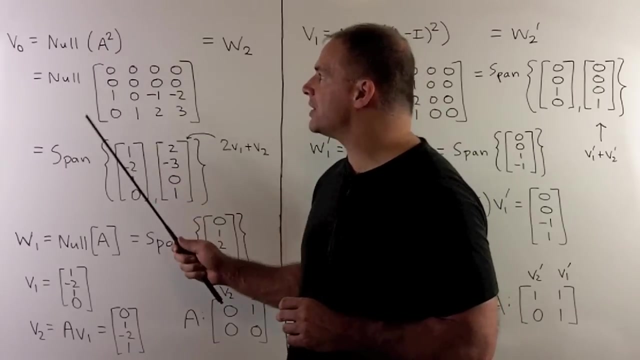 The tricky part. we want to find the basis that gets us from our A to our Jordan form. Let's find our basis First: eigenvalue 0. So V0 is equal to the null space, A minus CI, to the exponent of the minimal polynomial. 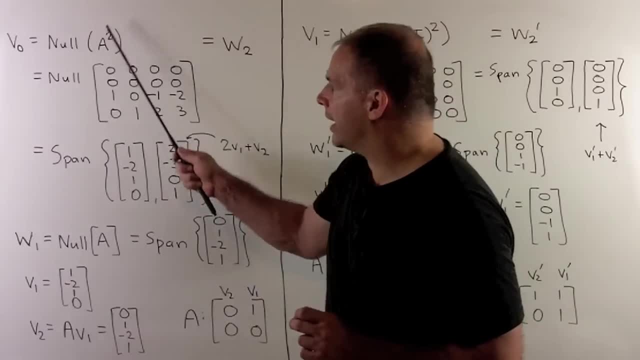 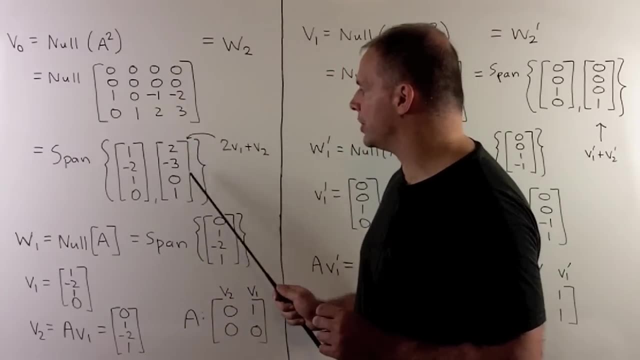 So that's A squared. If we work out A squared, we get this matrix. Its null space is given by the span of 1 minus 2, 1, 0, 2 minus 3, 0, 1.. 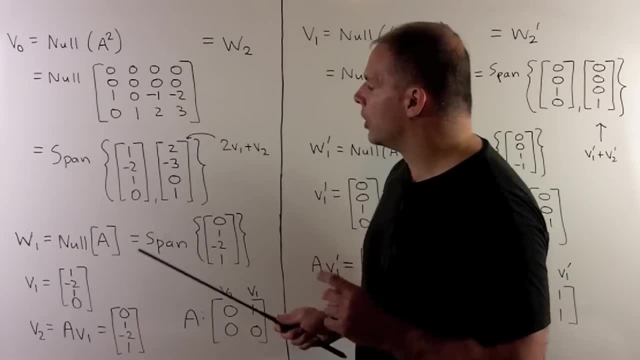 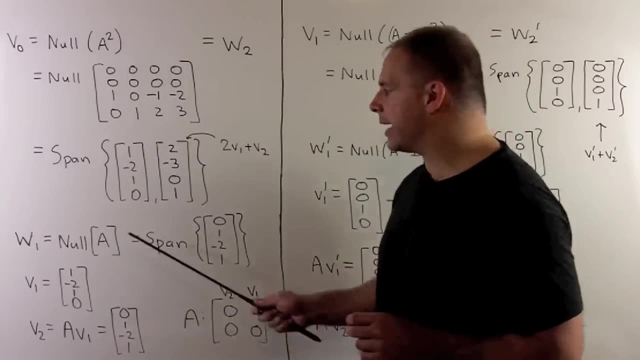 So that's going to be our W2.. For W1, we want the null space of A minus CI to the first power, which is just the null space of A That's given by the span of 0, 1 minus 2, 1.. 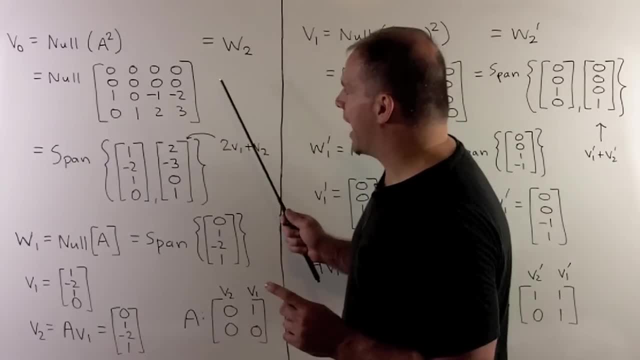 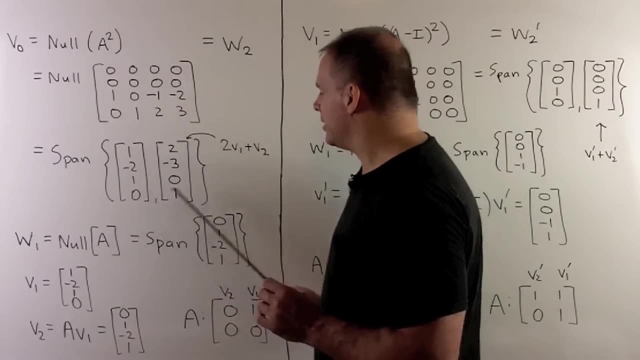 Now thing to note. we want to check. So if I apply this matrix to each of these vectors, we get 0 to come out. If I apply A to this vector, we expect 0 to come out. In this case, that's going to mean this vector. 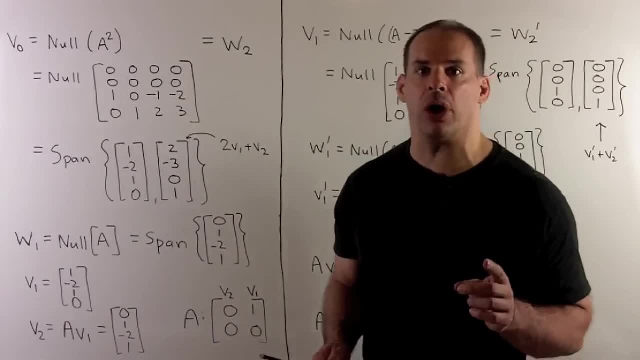 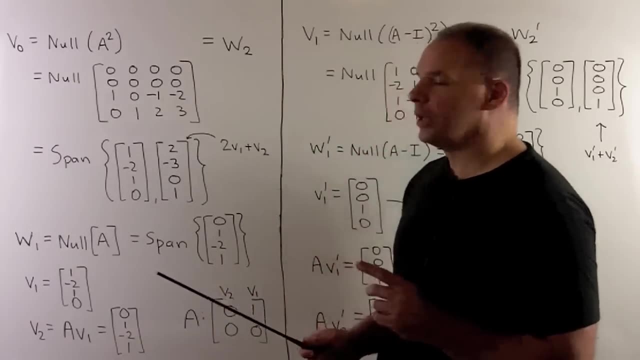 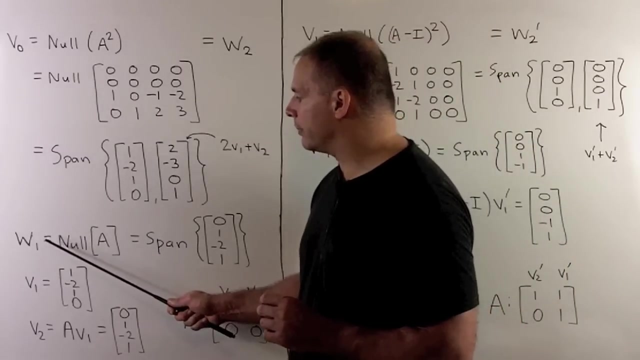 is an eigenvector for A with eigenvalue 0. So expect that for W1.. Now to find the basis that gives us our Jordan block, we take any vector in W2 that's not in W1. The only way I can be in W1 is if I'm a multiple of this vector here. 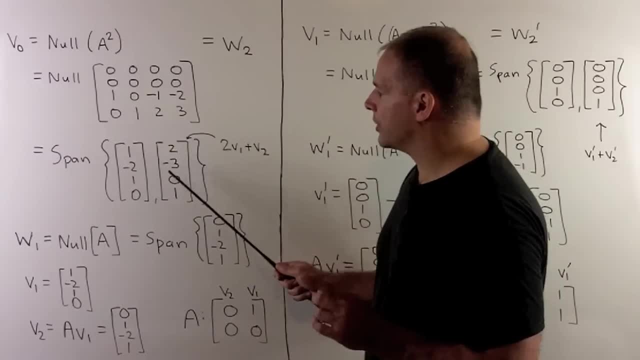 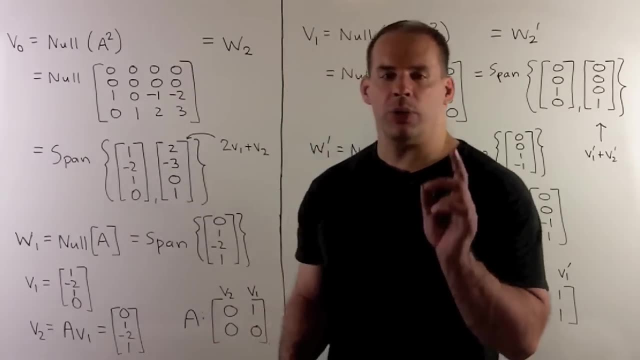 So either of these vectors will do. So I'll take the first vector. So V1 is 1 minus 2, 1, 0.. To get V2, we apply A minus CI. So we're just going to apply A. 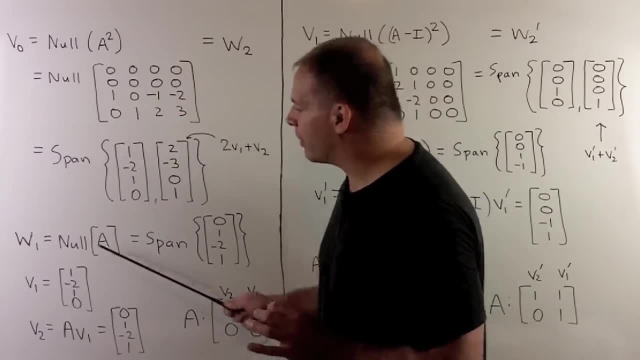 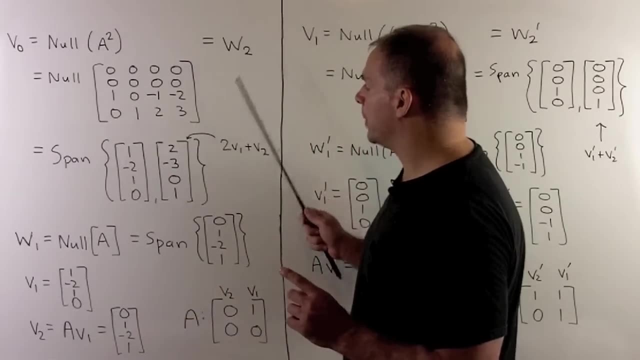 That's going to give us 0, 1 minus 2, 1.. So we have our basis. that gives us the Jordan block. Now note: this is still going to be spanning W2, because 2 minus 3, 0, 1 can be written as 2V1 plus V2.. 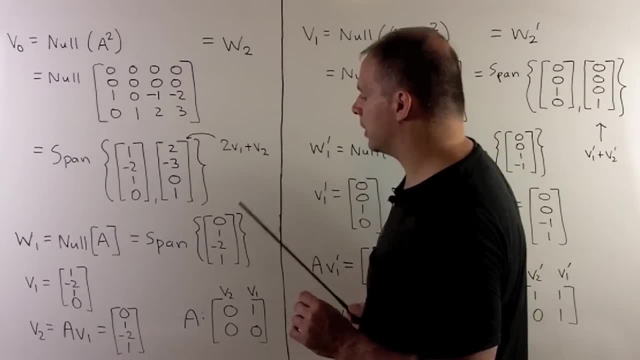 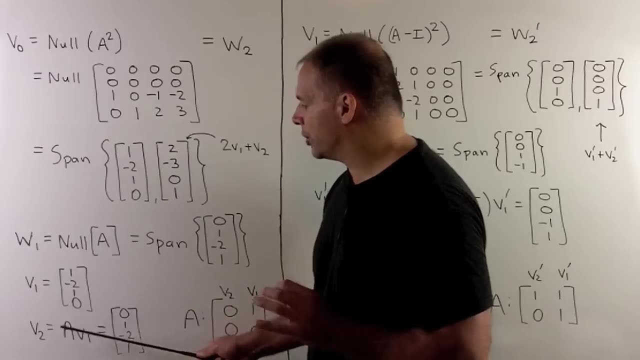 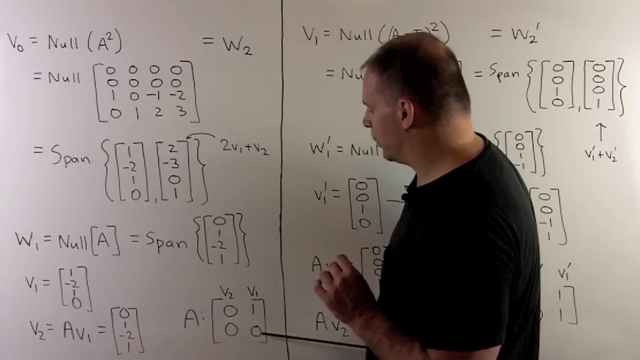 So that's another check on my work. Now, what does A look like with respect to this basis? Well, A of V1 is going to go to V2.. So that means, for the column that goes with V1, the coefficient of V1 is 0. 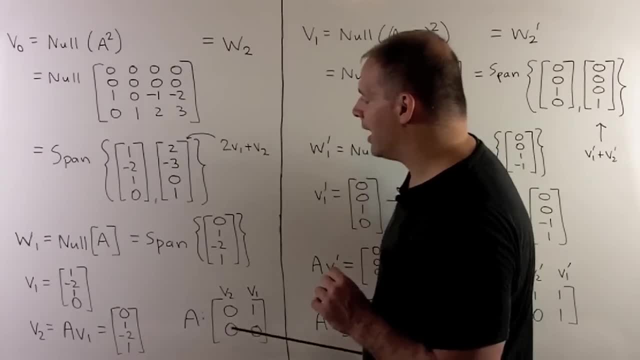 The coefficient of V2 is 1.. A is going to send V2 to 0. It's in the null space of A, So we're going to have a 0 and a 0. So this is going to be our Jordan block. 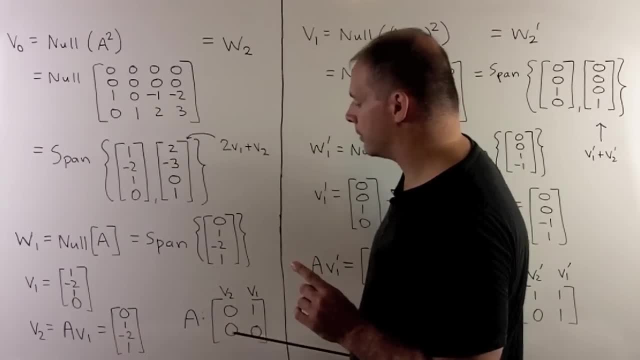 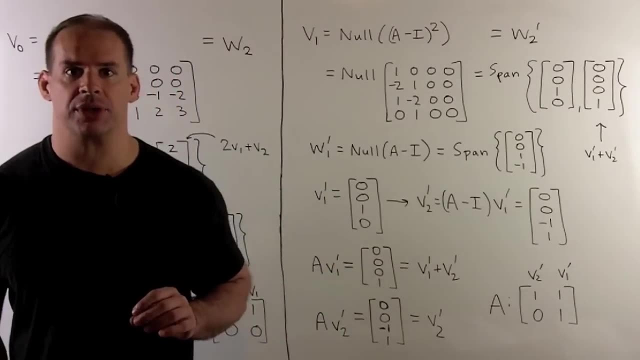 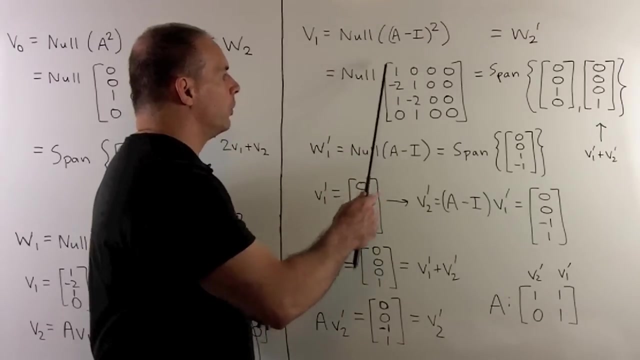 That goes with eigenvalue 0.. Now for eigenvalue 1, same procedure, just a few extra steps. For V1, we use the null space of A minus I squared, So we get this matrix. here We find its null space. 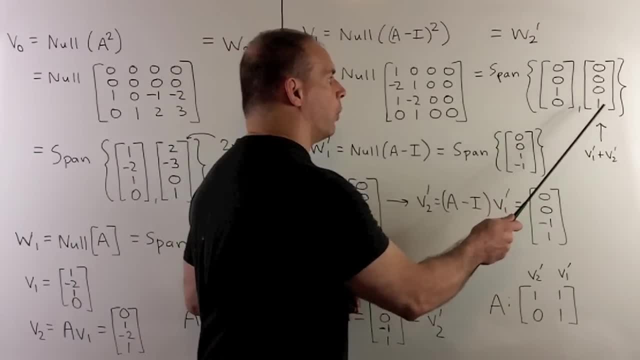 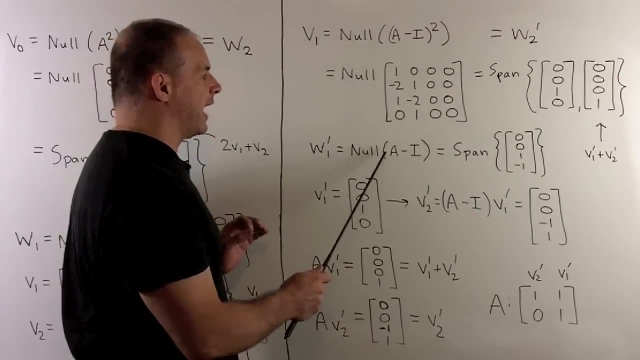 That's given by the span of 0, 0, 1, 0 and 0, 0, 0, 1.. So that's going to be our W2 prime. For W1 prime I use the null space of A minus I. 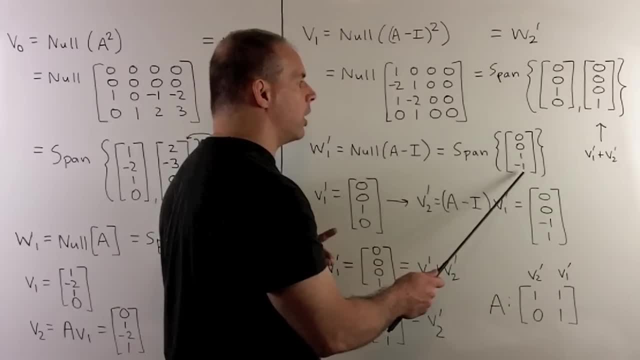 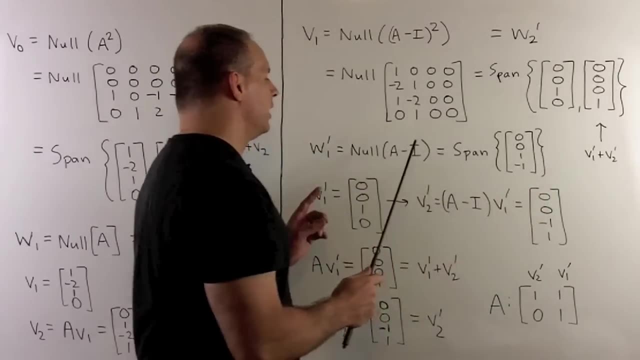 That'll be given by the span of 0, 0, 1, minus 1.. Okay, again we check. We apply this matrix to each of these vectors, We get 0.. Here, if I apply A to this vector, 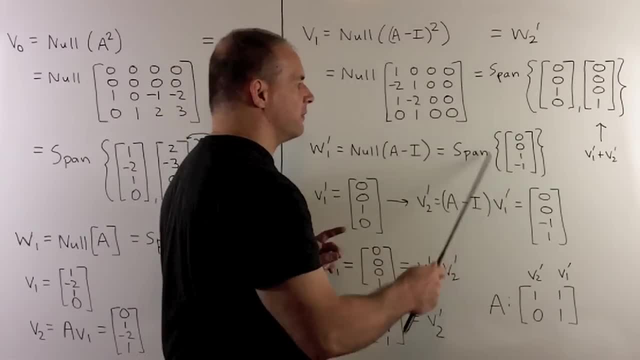 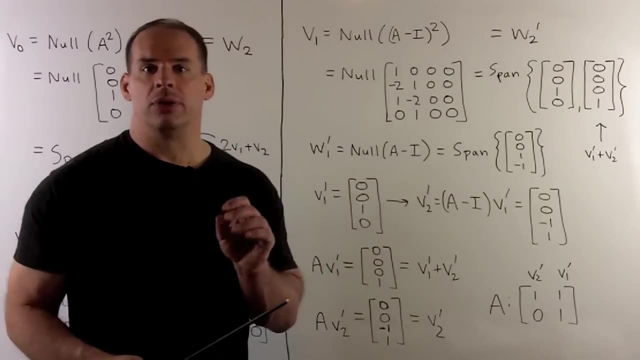 since we have eigenvalue 1, we expect to get this vector back And we do So that's our check Now to find the basis for the Jordan block. I find this. I find any vector in W2 prime. 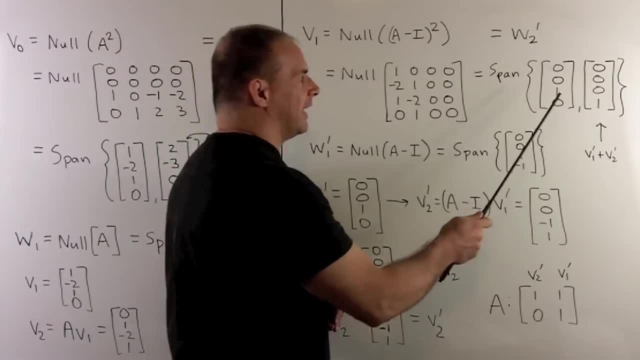 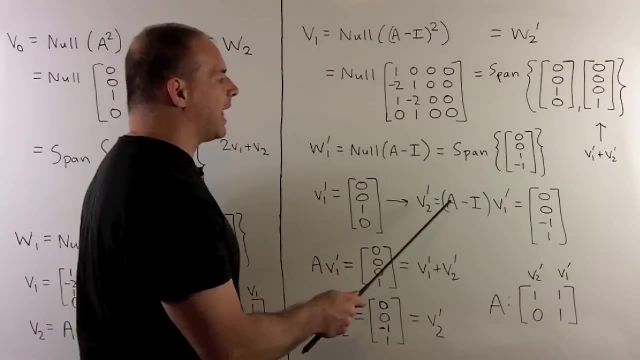 It's not in W1 prime, Okay again, either of these vectors will do So we take the first one, So it's our V1 prime. To get V2 prime, we apply A minus I. That gives me 0, 0, minus 1, 1.. 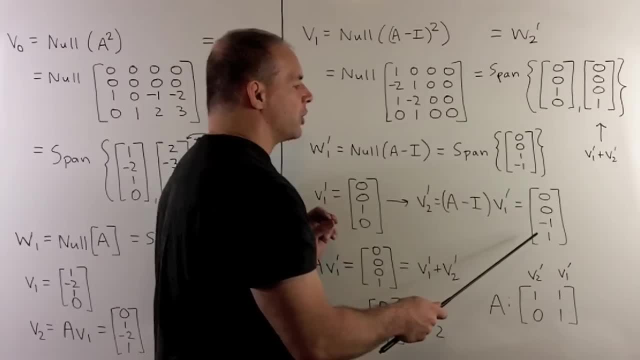 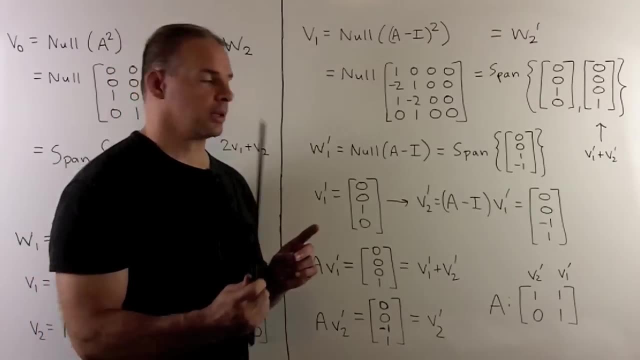 And we know it's a multiple of this vector, So it's going to be an eigenvector for eigenvalue 1.. Okay, and again we're in W1 prime, So that's expected Now if we want to see what our Jordan block looks like. 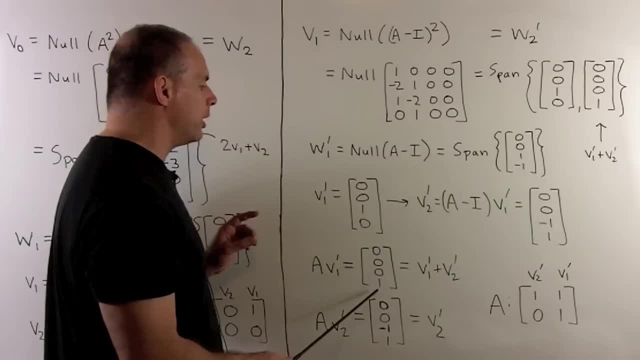 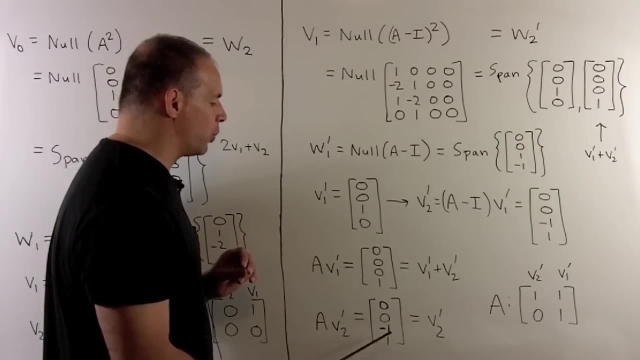 okay. if I apply A to V1 prime, we get 0, 0, 0, 1, which is V1 prime plus V2 prime. If I apply A to V2 prime, we get 0, 0, minus 1, 1.. 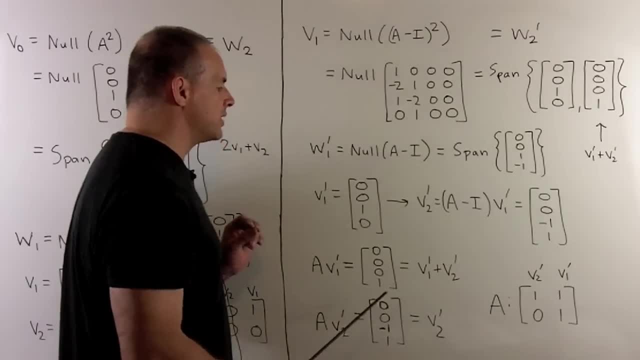 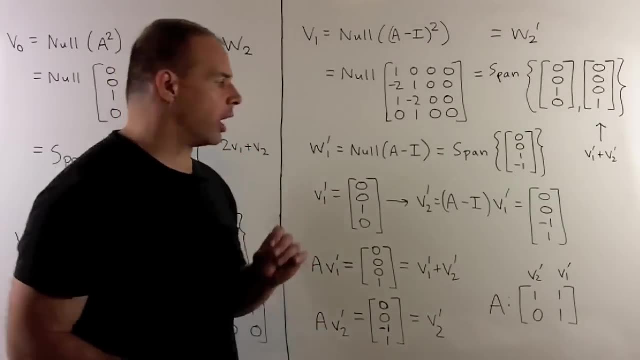 And that's our V2 prime. So when we set up our block for A V1 prime goes to V1 prime plus V2 prime. So both coefficients are 1.. So I have a 1 and a 1.. 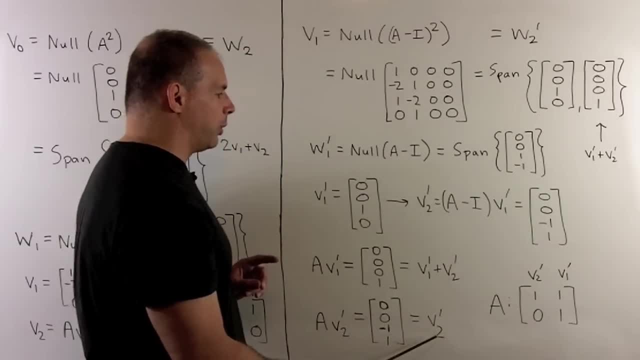 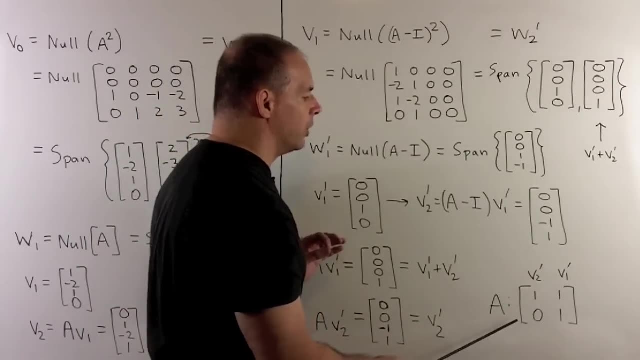 For V2 prime we're going to go to V2 prime itself. So that means coefficient for V2 prime is 1.. For V1 prime it's 0.. So we note, here we have our Jordan block for eigenvalue 1.. 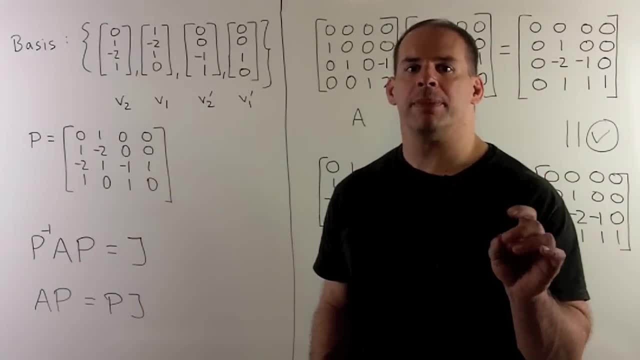 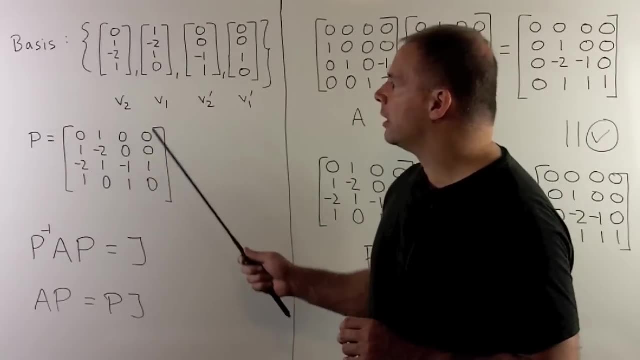 Now that we have our basis, we can find the matrix P that carries A to the Jordan form by conjugation. So we get our matrix P. We're taking our basis vectors, We load them in as the column vectors of our P. 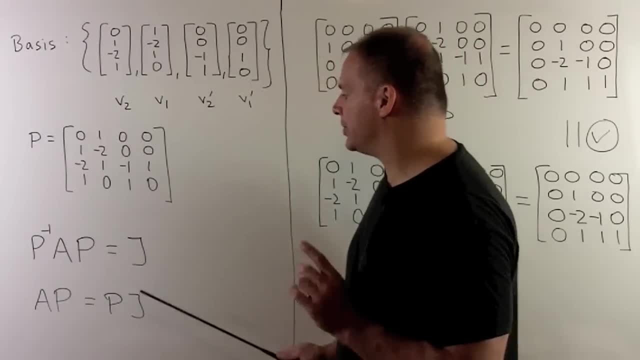 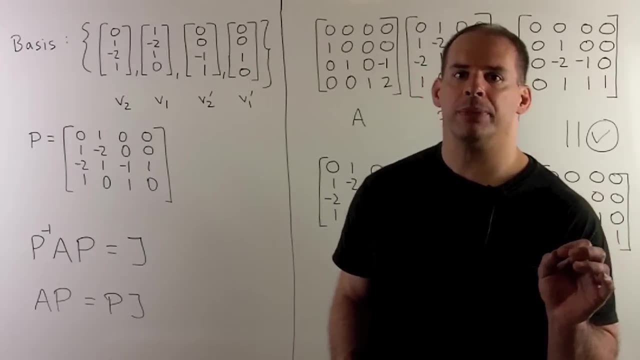 Then the relation is P inverse A. P is equal to our Jordan form J. Now for here. we're just interested in checking our work, So I don't want to invert our matrix P. It's 4 by 4, so that takes some work.